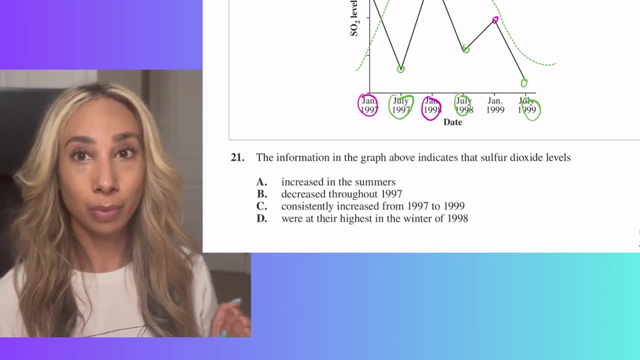 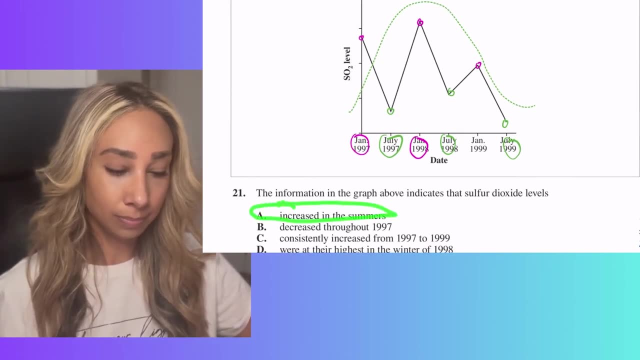 carbon dioxide levels are. So this is one of those questions where you want to choose the most, the best answer, the one that's the most applicable. So did we increase in the summer? No, we talked about that, And in the summer we actually decreased. So that doesn't work. 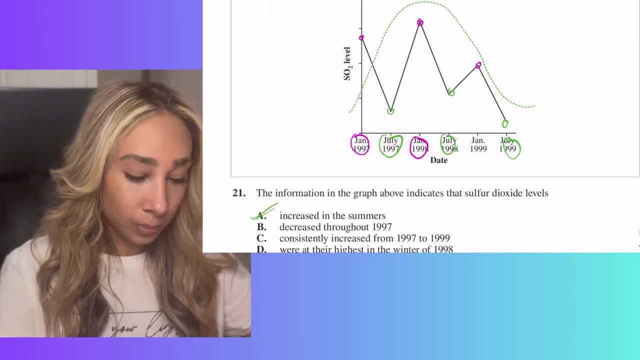 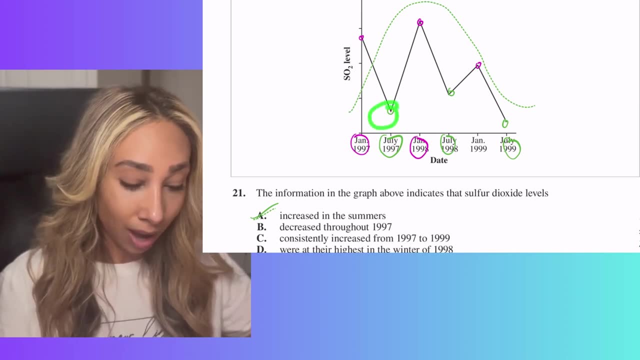 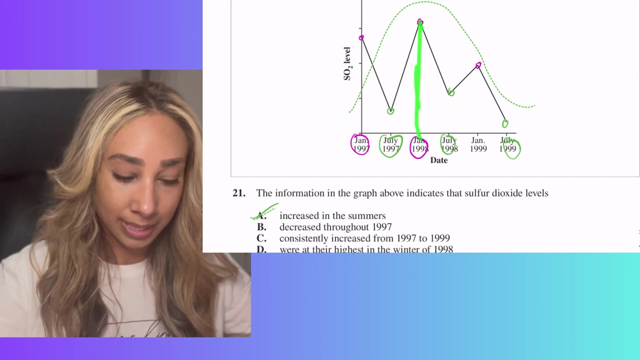 Did we decrease? Did we decrease throughout 1997?? Um, not really. I mean, we did in just July, but not all of 1997, right, It's kind of goes up a little bit before we hit January of 1998.. This portion here would still be 1997.. It. 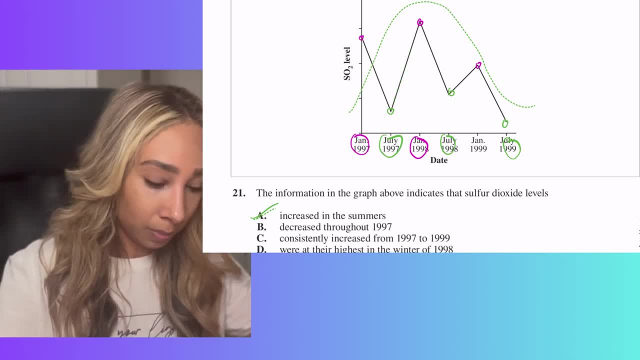 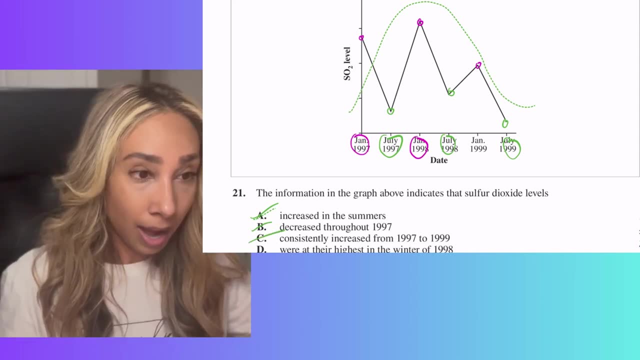 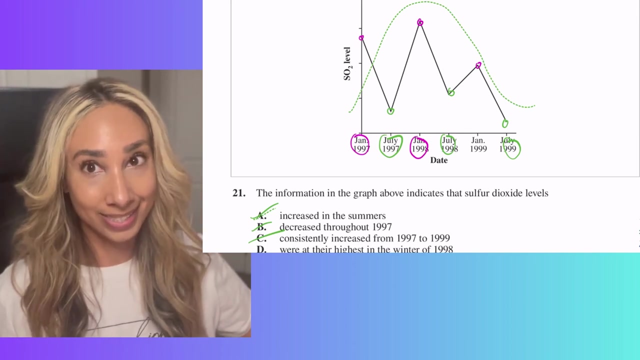 would just be the fall of 1997.. So that one's not going to work for us. Consistently increased- Well, we just talked about that with our overall trend. That didn't happen. That leaves us with option D. So let's verify that They were at their highest in the winter of 1998.. Yes, we can see that peak. 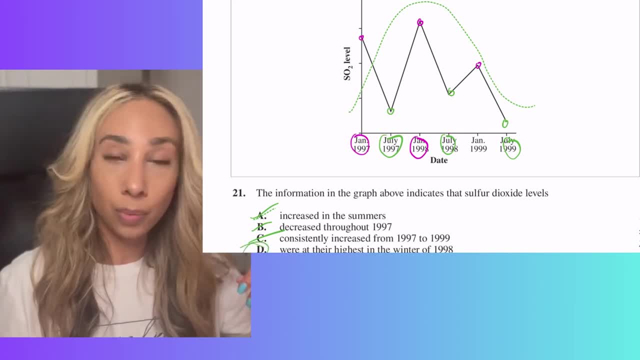 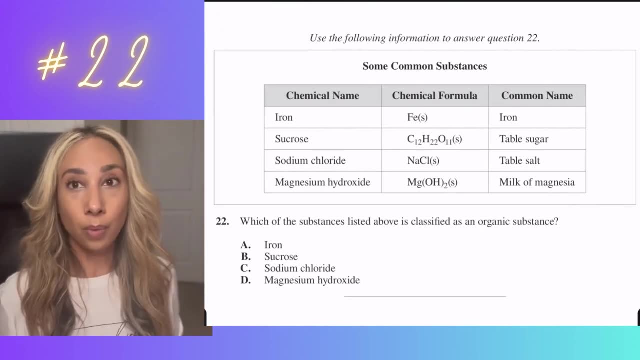 right up here, It's definitely at its highest, So that's going to be our best option. Okay, Number 22.. So this one is really asking us if we understand what an organic substance is. And now I don't mean organic like organic farmer's market, I mean organic in the chemistry. 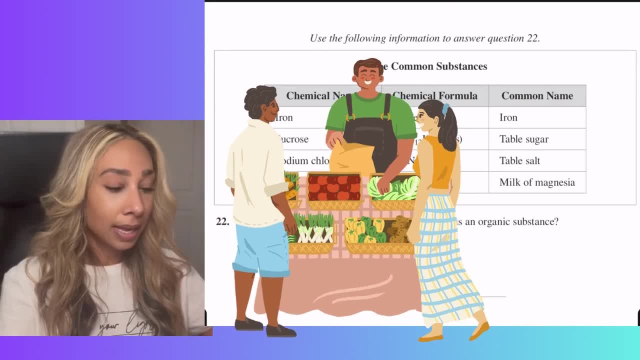 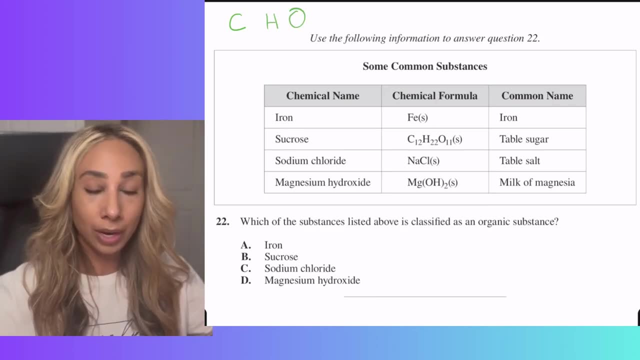 sense. So for something to be organic in the chemistry sense, it's going to be made up of carbon hydrogens and sometimes oxygens, just not always. So now we can go ahead and look at our list and see which one of those would be organic compounds. Well, iron's a metal. 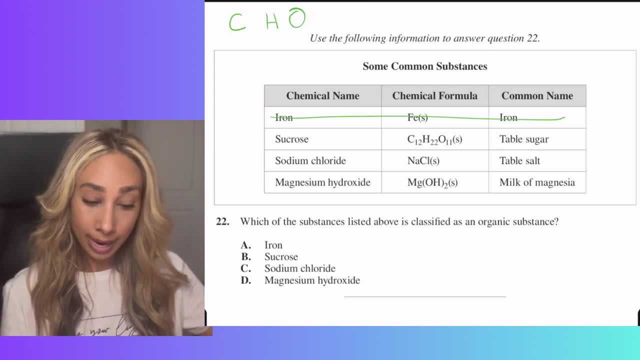 so that's not going to work. Um sucrose looks like it has it. It has everything I mentioned above, So we'll keep that on the in the list. Sodium chloride: It's got sodium in it. That's a metal. Magnesium hydroxide: It also has magnesium. That's also. 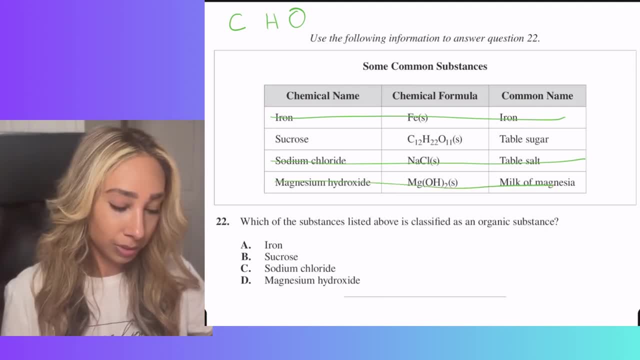 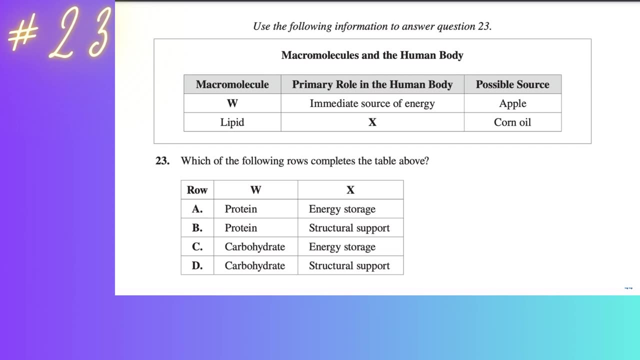 a metal, So our best option for this one is going to be sucrose, which is really just the sugar that you all probably consume on a daily basis. Okay, 23.. Sorry, I had some technical difficulties, but let's look at 23.. So what they're really asking you is, first of all, do you know what? 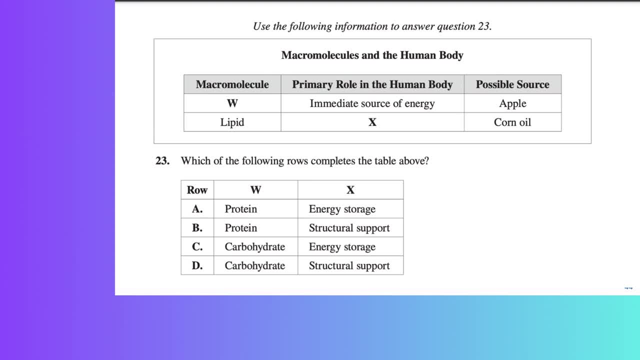 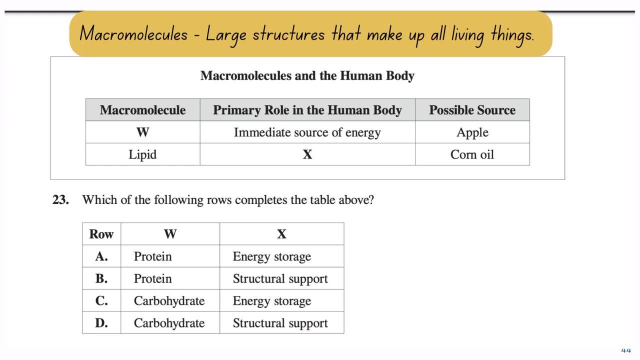 macromolecules are, and do you know the roles that they play inside our body? So macromolecules, just like I said here, are large structures that make up all living organisms. So there's four of those, and those are going to be our carbohydrates, lipids, proteins and nucleic. 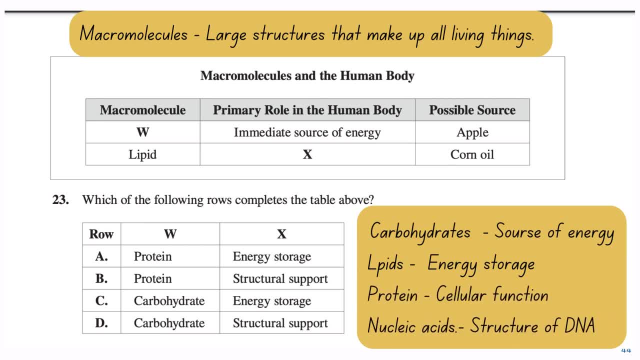 acids. So your job is to know in a general sense of what these are, what these are. So carbohydrates: often when we think of them we think of bread and we think of a food that sometimes has a bad rep in our society. But carbohydrates, really what they are is their. 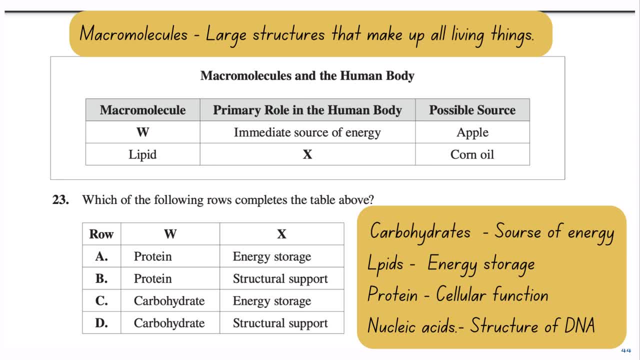 main source of energy, And they're not just found in bread. They are found in things like plants and earth. They are found in plants, so things like fruits and vegetables, But the main thing is our body breaks it down into energy that we can use right away. There's just different kinds and certain 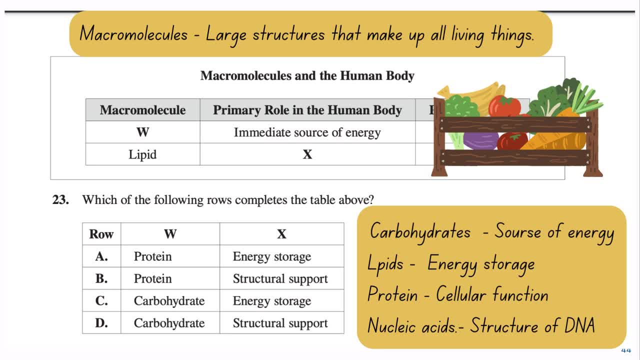 kinds are not as good for you as other kinds, right? So that's kind of what that is. Lipids, on the other hand, they are fantastic for energy storage. as well as forming the membranes of a cell. Proteins are involved in nearly all of our cells, So they're not just found in bread, they're found in. 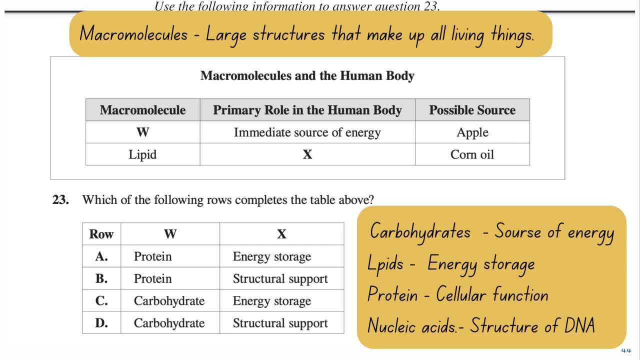 all cellular functions. They are used for structural support as well as moving things from one part of the cell to another part of the cell or even parts of the body. Our last one that we have is our nucleic acids, And you might remember this. These are going to help build. they are the 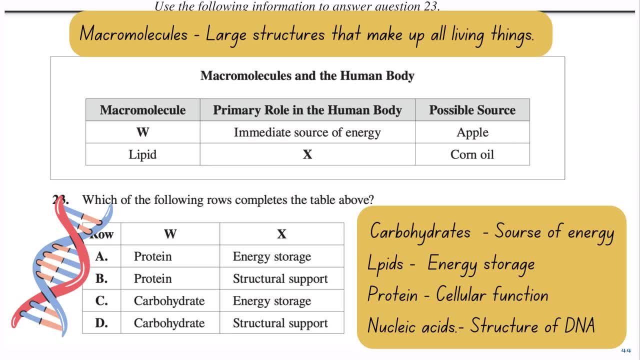 building blocks of DNA, and they actually are the parts of the rungs of the ladder that make up DNA. So what we need to do is decide which macromolecule is an immediate source of energy, and it's possibly coming from an apple. 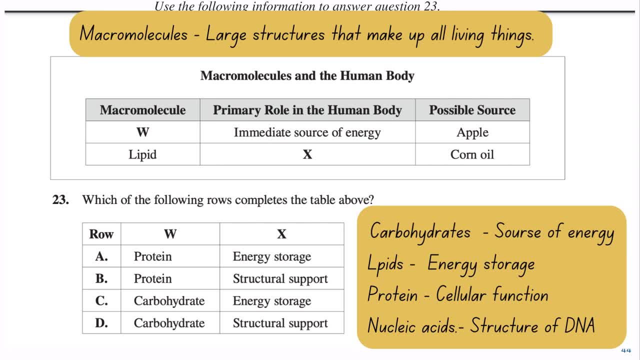 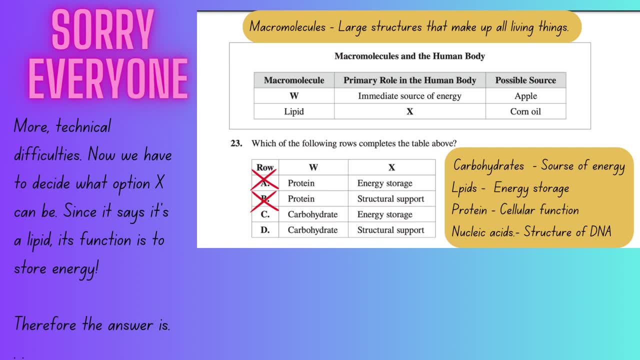 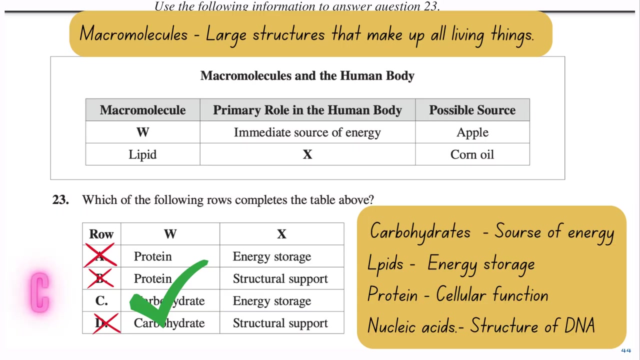 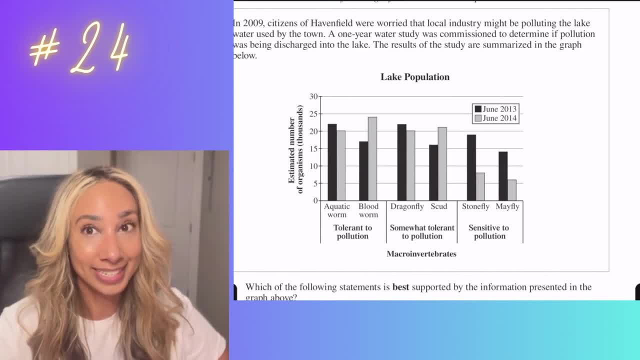 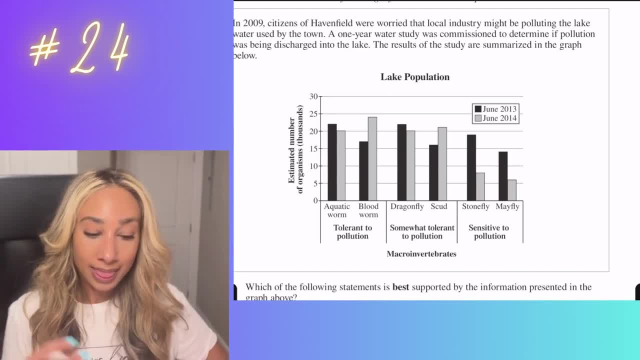 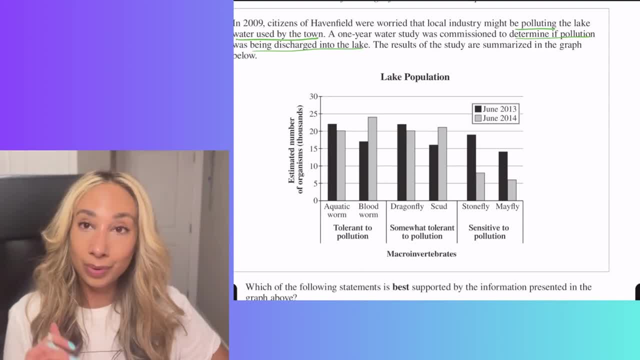 Okay, 24.. Okay, 24.. Sure, okay, Okay, 24 minutes and a half. So we're going to tonightAKEL experiences method, So let's just make them quick. Okay, There, hey. So one of the things that are probably going to be our best indicators is going to be our indicator species. 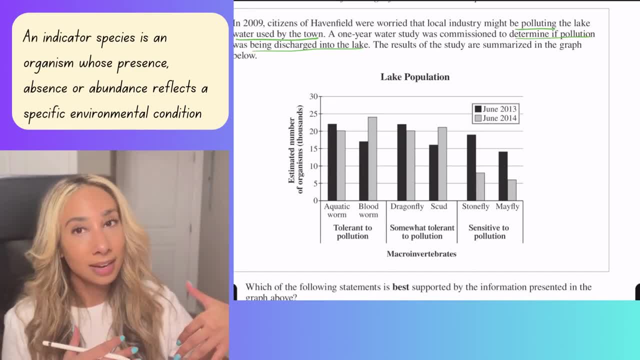 Now, some of you might have done the field trip to the river, at least I guess in southern Alberta. I'm not too sure. I think northern Alberta has a slightly different. Yeah, northern Alberta should have a different field trip, but regardless, you're looking at species and 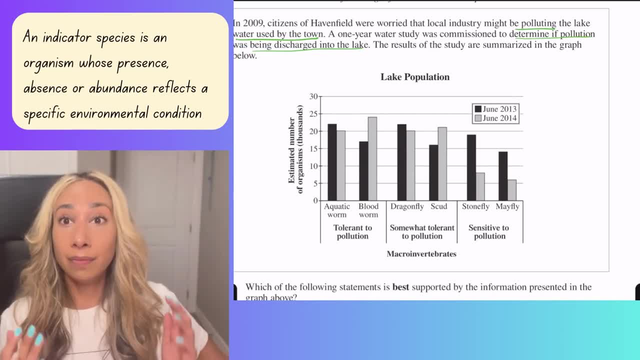 How those presence of species can tell us if the environment that they're living in is healthy or not. So one of the ones I'm noticing right now is our stonefly and mayfly. those species are so sensitive to any changes in water that they're not going to survive if the change is even just as subtle as 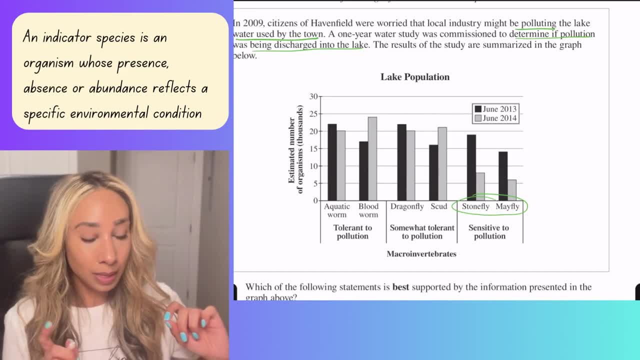 Like a point, something in pH. So that's something to keep in mind. Now Let's see what's happening here. We've got our worms. Well, it says: our worm, our worms in general are tolerant to pollution. But what we do notice is that there is a little bit of a dip here and then all of a sudden there's an increase here. 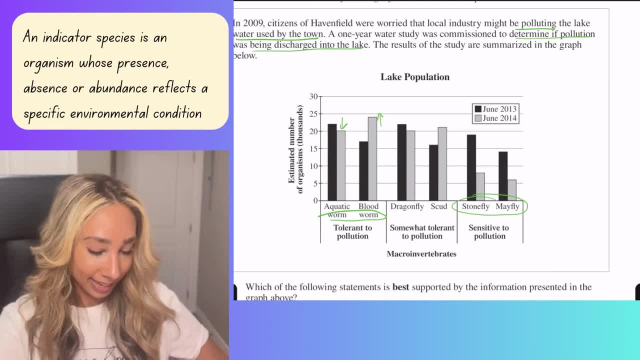 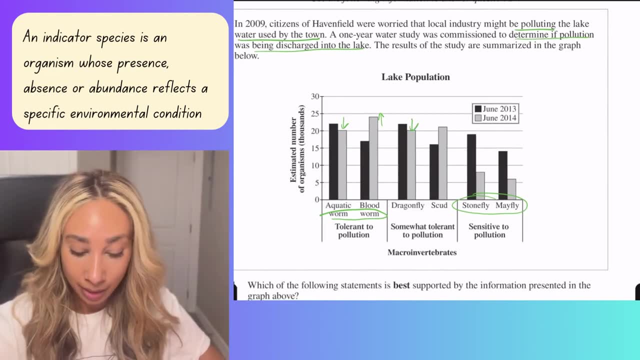 So that's something to consider. The dragonfly and scud- I think that's how you say- that the dragonfly and the scud are somewhat tolerant, But we also notice there's a decrease in the dragonfly Population. we look at our stonefly and mayfly. They're extremely sensitive again. 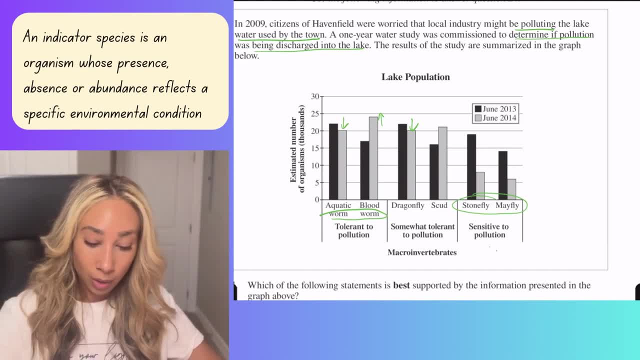 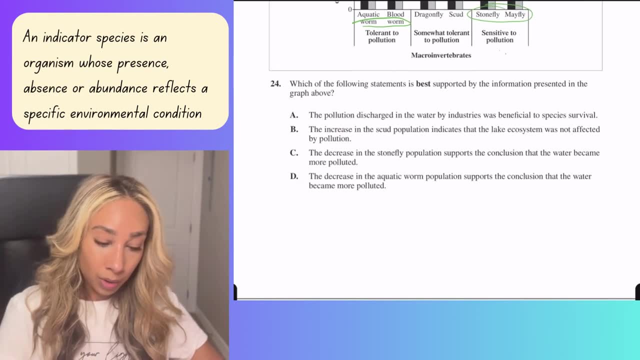 Really good indicator species, because they're gonna tell us if something's wrong. Well, They really decrease there. So that's gonna tell us something for sure. So let's read our question. We want to know which of the following statement is best supported by the information presented in the graph. 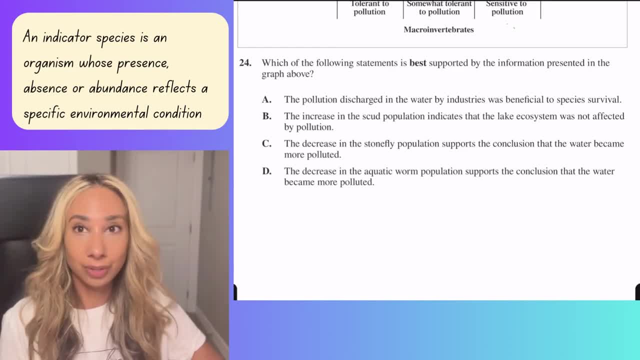 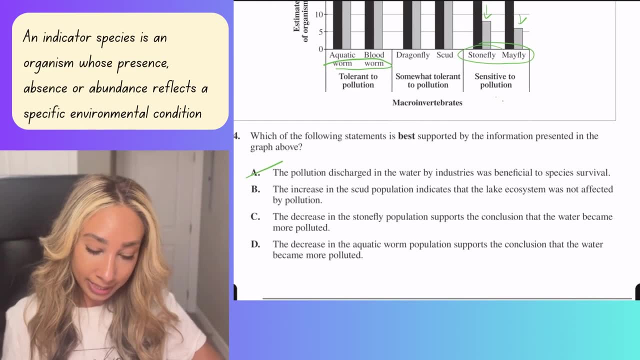 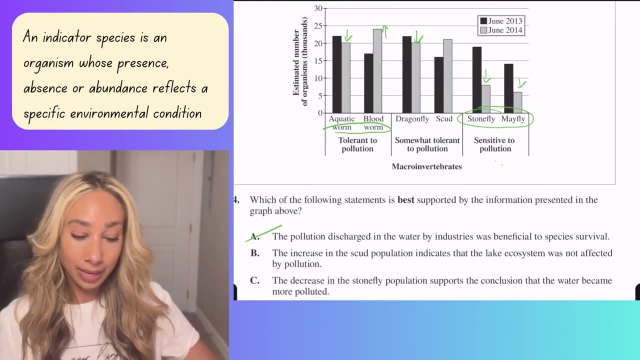 so Pollution discharged by the water industry was beneficial. It wasn't beneficial because some of the organisms decreased. Letter B- the scud population, indicates the ecosystem was not affected. That is true in the sense of like, the scud population increased. But because we're talking about an ecosystem, we need to consider all the other organisms present. 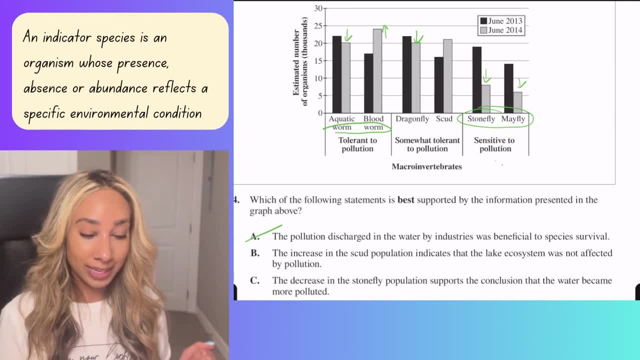 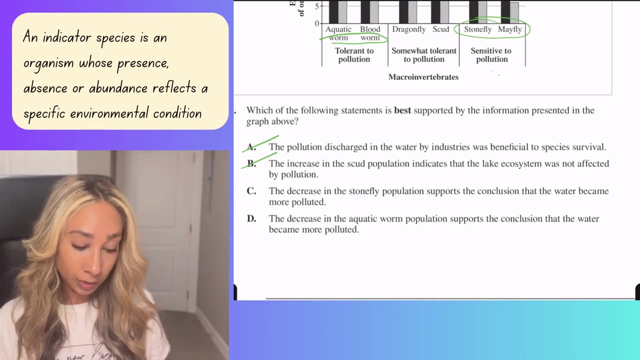 Based on the fact that other organisms had a definite decrease. it's not going to be beneficial because other organisms are perishing at the expense of another or at the expense of this pollutant. Okay, C, Let's see The decreased stonefly population supports the conclusion. 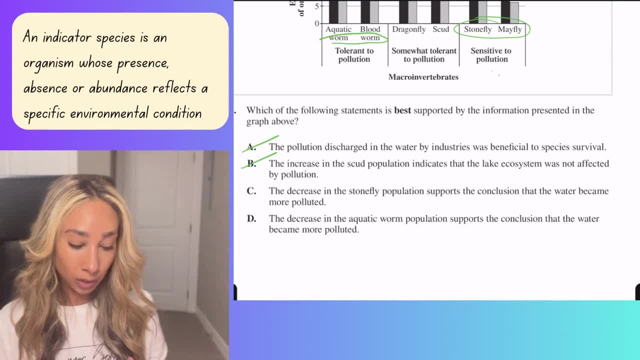 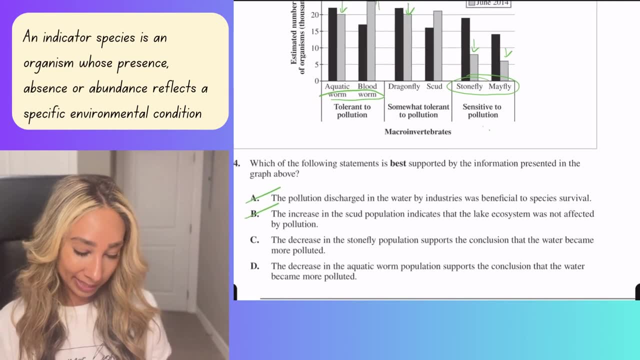 Yeah, that one's probably going to be our best bet. Let's look at D. The decreased aquatic worm population supports the conclusion that the water became more populated or more polluted, Sorry. So let's see, I would say yes for this one. 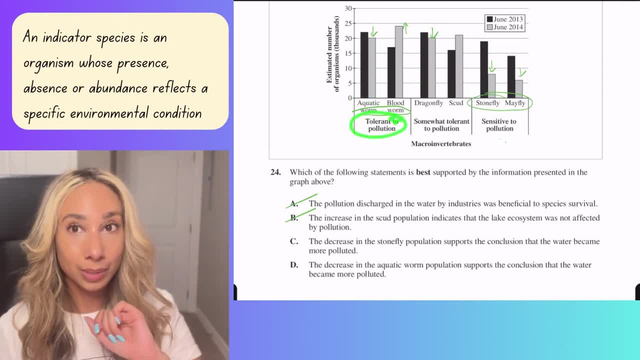 However, because the worm population is tolerant to pollution, you can't really use that to best support. So if you were trying to like- let's say, debate about this- to someone to say whether or not the water is polluted or not, it's going to be a little tricky to say that because it's tolerant, meaning it can survive some of those changes. 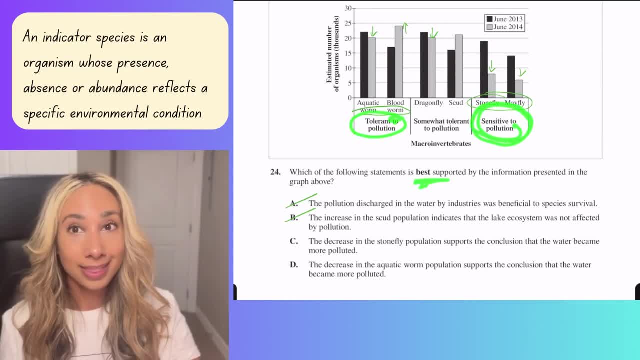 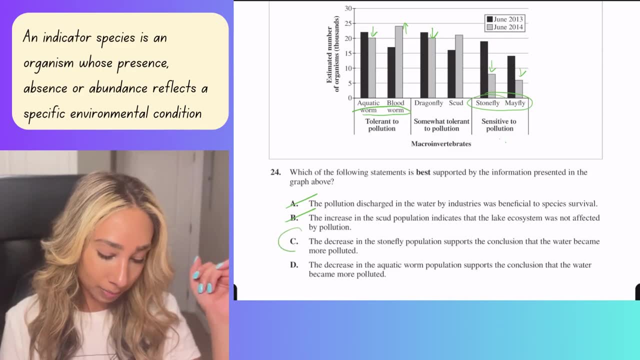 But our Indicator species, These ones here, they, like I said, any small subtle change and they're not going to be able to survive. So our best answer for this one is definitely going to be C, Okay, 25.. 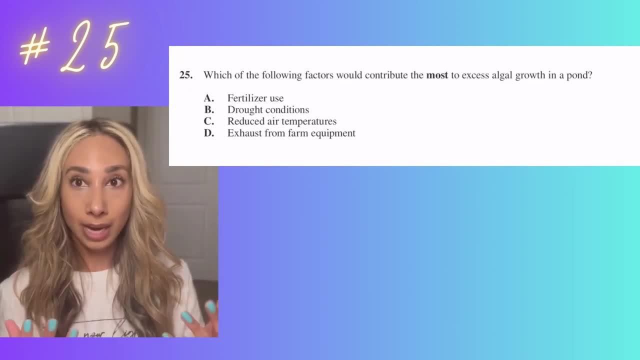 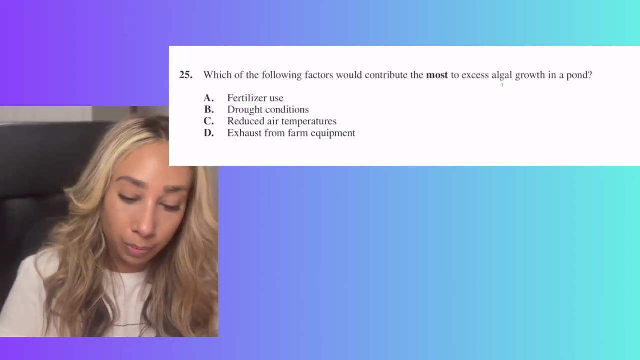 So this is another one where you need to think about what's happening in terms of other aspects of the environment. So we're looking at algal growth, So algae growth requires a couple of things. So they photosynthesize. 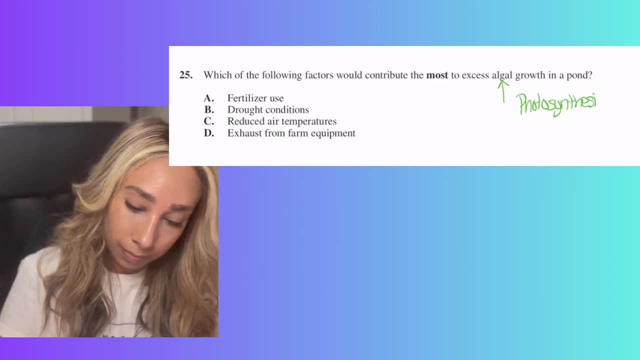 But when they also photosynthesize, they need nutrients, And those nutrients are normally going to be in the form of nitrogen and phosphorus. Well, if they photosynthesize, there's a couple of things that are going to make a difference. 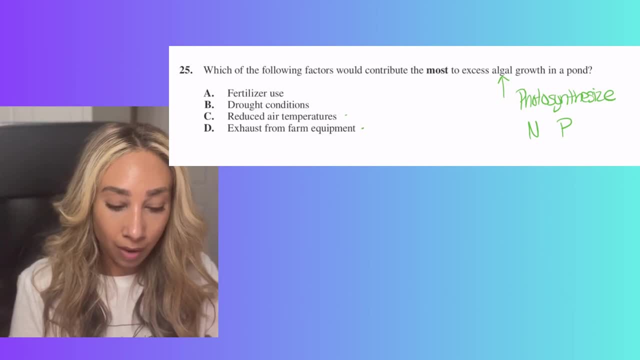 The air temperature could make a difference- Exhaust from a farm equipment could, But algae grows in water, So we're thinking about ways the water can be impacted that will impact its growth. So one of the things that we can really think about is going to be our fertilizer. 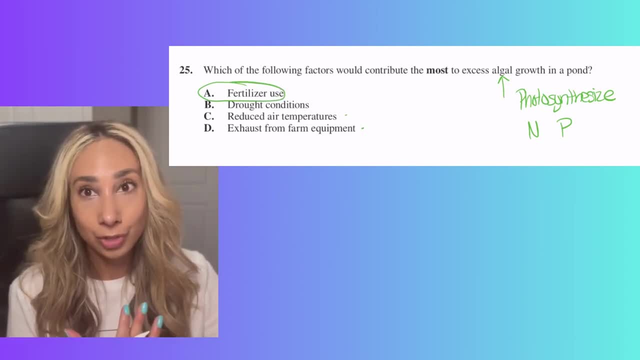 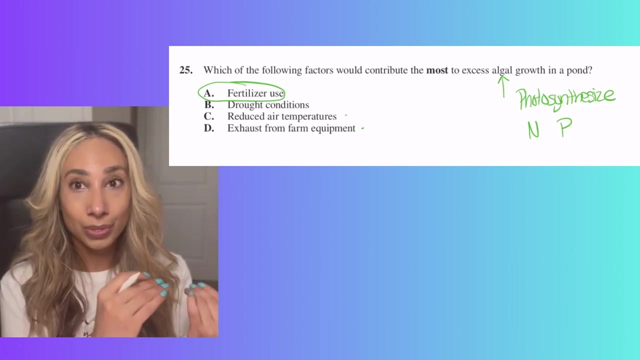 And this is one where you honestly need to go over that nitrogen cycle if you're not familiar with it. So what happens is, with the fertilizer, all the nitrogen is used to help make grasses and plants grow, But as water comes by and hits the soil, that water carries over the nutrients from the fertilizer into places that are heavily bodied water. 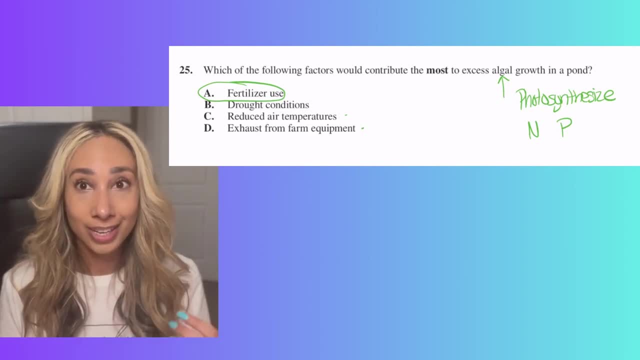 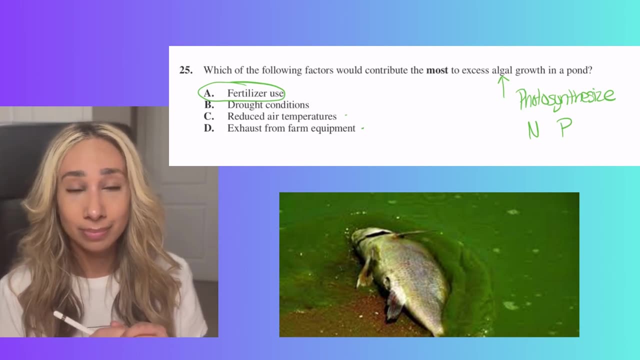 Which means things like algae. They can grow and kind of take over. In fact, they take over so much of the water. They actually do that to fish, which is really really sad, in my opinion. Okay, number three: we're looking at toxins. 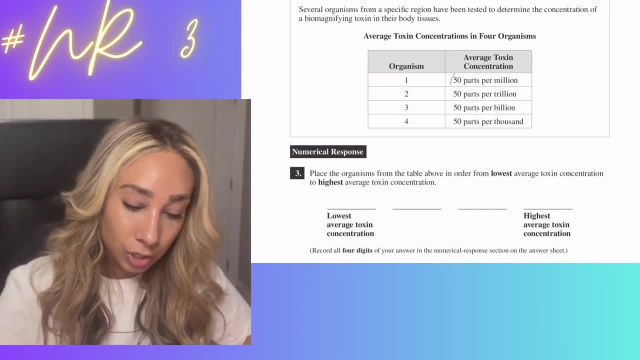 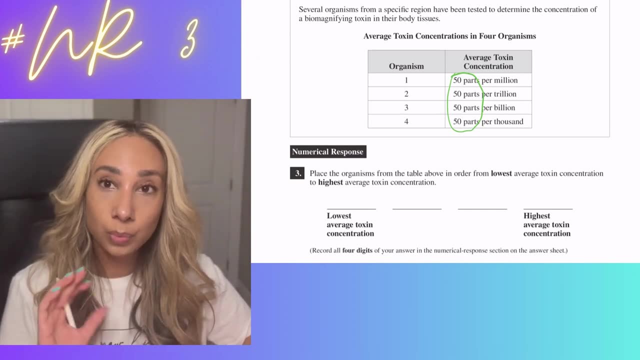 So the best way I can describe this one is the toxin. that number is the same: It's 50 parts. So that's great, But what's tricky about this one is we've changed the denominator, if you will, So I'm going to break it down into small numbers. 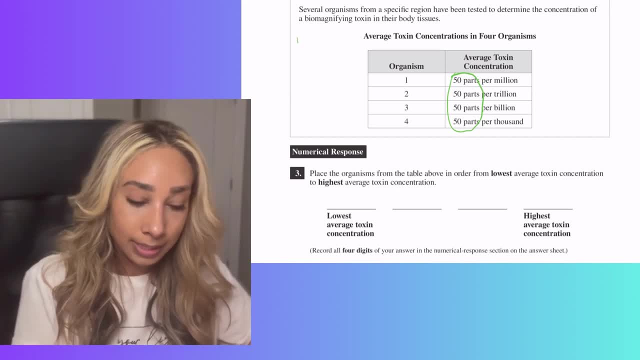 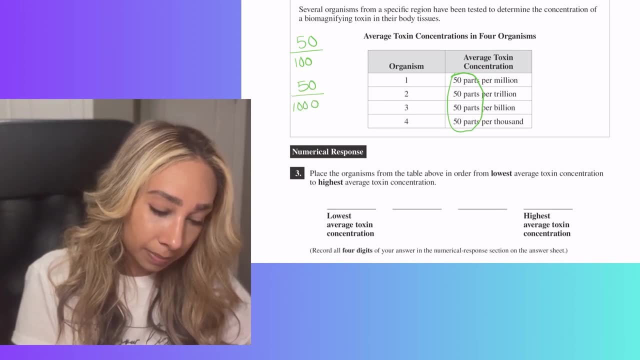 And then we'll look at the places I'll use for the numbers that are on here. So let's say we had 50 out of 100.. We had 50 over 1,000. And we had 50 over 10,000.. 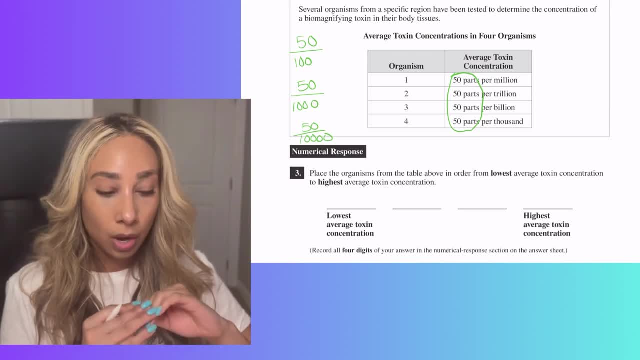 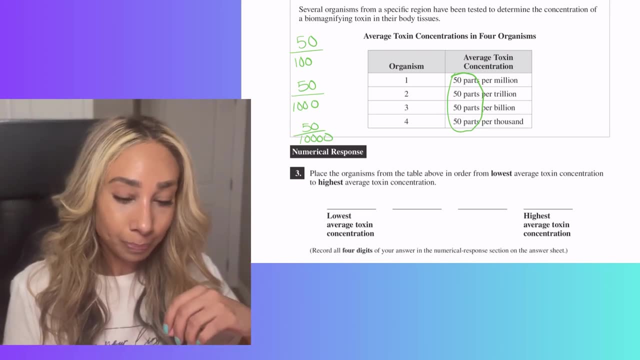 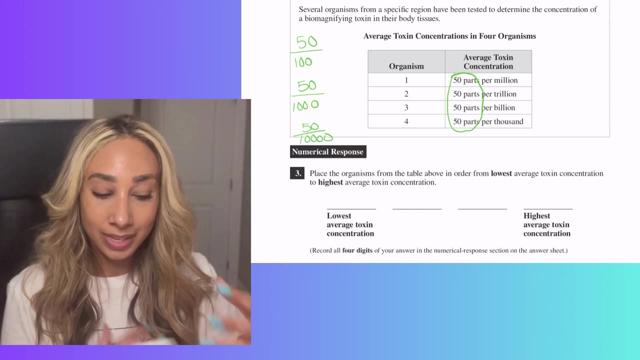 So because we're talking about a toxin, we're going to want the smallest number of toxins present, right? So the first example I gave us, That's about 50%. Half of the substance you're looking at is made out of toxins. 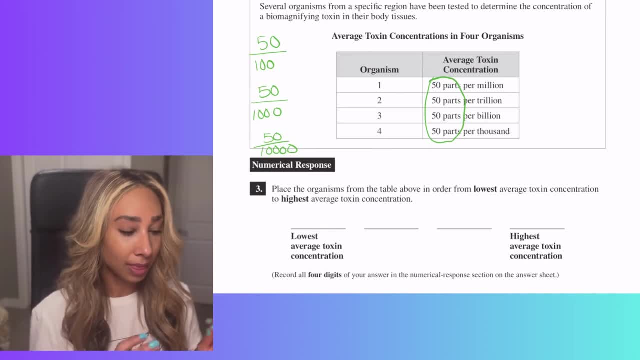 In this one here it's a little less, because your toxin, the part of it, the part of the toxin, is 50. But the whole of it is 1,000. And then in our next example, the 50 over 10,000, well, it's getting. there's less toxin per the whole. 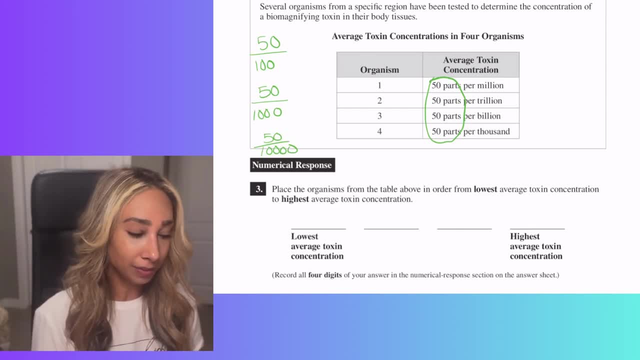 Or the other way I can describe it is like we're diluting it. Here's a 50% mixture, Here's we're diluting it by 10 times, And then here we're diluting it by another 10 times. So, in terms of toxicity, you want the ones that is most diluted, right? 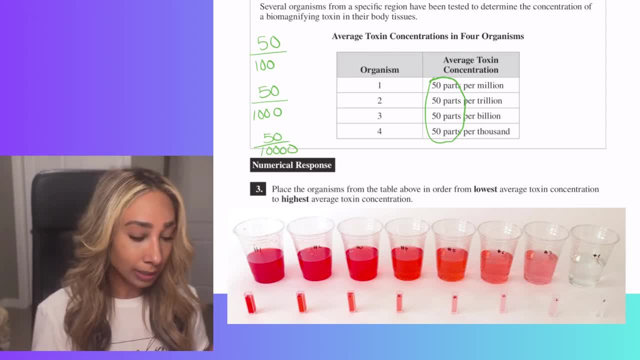 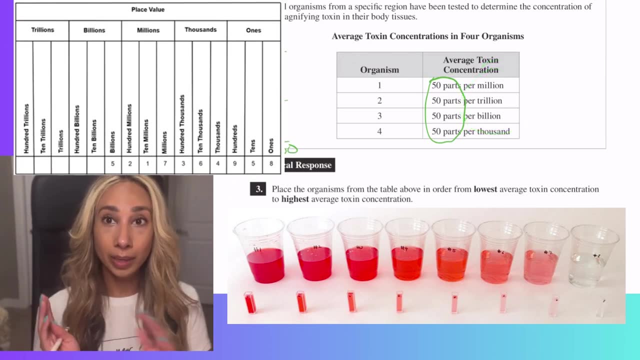 We want the one that has the least amount of toxins in here, So our lowest concentration will be the one with our largest place value. So I'm going to pop a place value chart there so we can see how we want to organize the order. 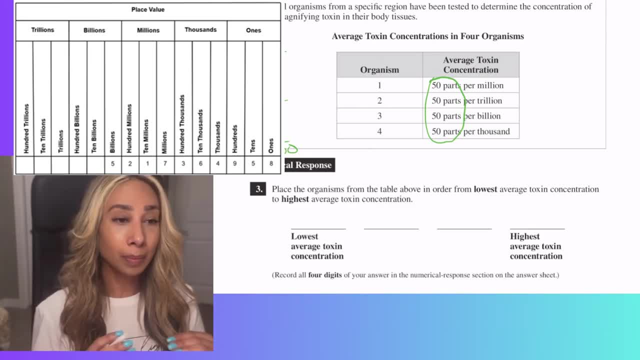 Some of the billions and trillions can get a little tricky, But our lowest toxin will be the one that is in the biggest part. So our biggest part is going to be our trillion. Then the next one is going to be our trillion. 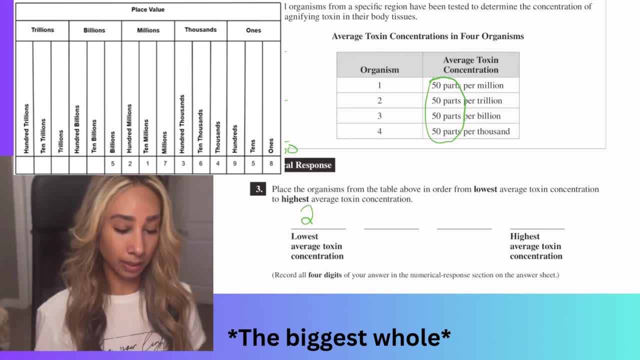 Then the next one is going to be our billion, The third will be our million And then the last will be the 1,000.. So we can organize it like that, and now we've got everything from our lowest concentrations to our highest concentration. 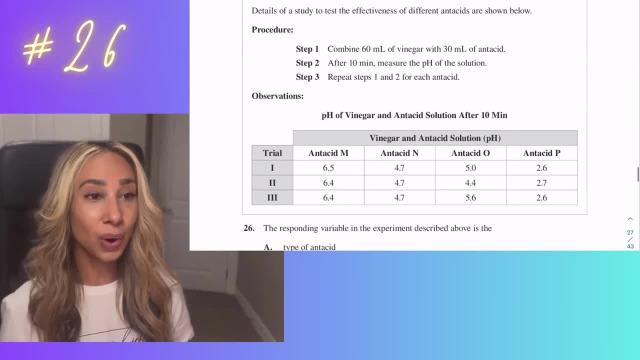 Okay, number 26.. So what we need to do here is we are looking at a couple different things. I'm going to read out that experiment and then we'll go through it. So what we're doing is we're looking at the effectiveness of anti- pronouns. 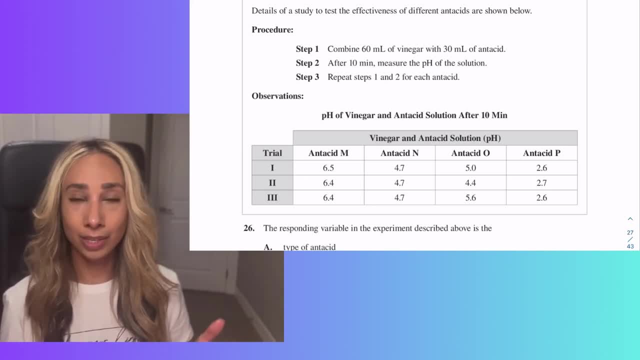 anti-acid. So anti-acids are things like Tums, Gaviscon, things that honestly, people take when they get really bad heartburn. What we're doing here is we've got our vinegar that's going to act as the acid and we're combining it with the anti-acid, which is the medicine Now normally. 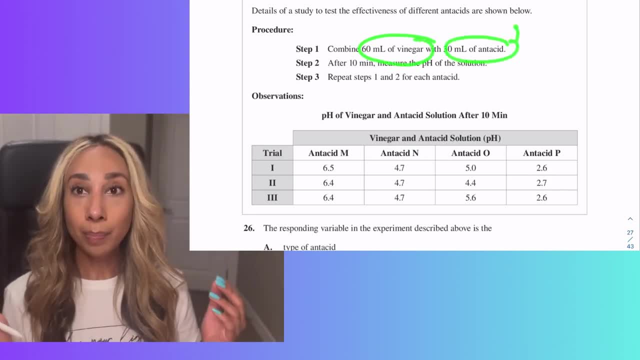 what's going to happen if you think about mixing an acidic solution with a basic solution. it should neutralize. In the case of a person that needs a heartburn, it should decrease. In the case of us, it's just neutralization, which I guess is both the same in both perspectives. The question is: 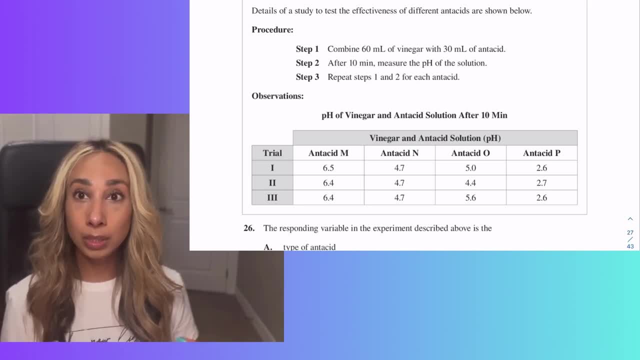 asking: we want to know what the responding variable is. So responding? think about that as response to something. So in the case of a science experiment, it's what we're measuring. Well, in this example here we are only really measuring the pH, So we're not measuring the type of anti-acid. 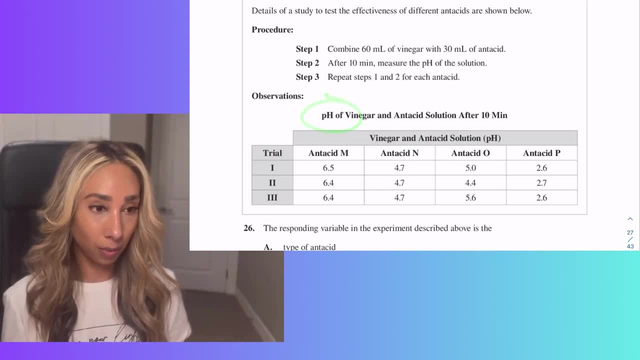 because we're using the same acid. we're using different anti-acids the whole time, but we're not measuring that. That's not what we're recording. That would be probably the answer to that question. So we're not measuring the type of anti-acid because we're 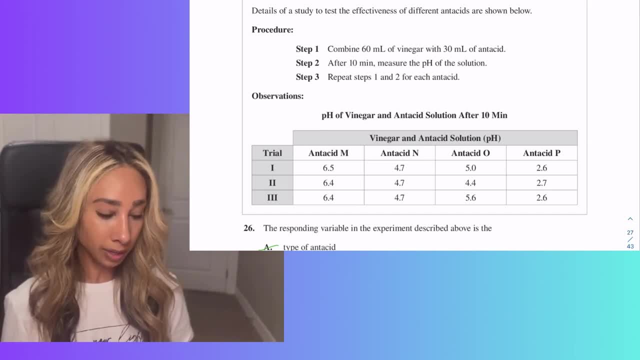 probably our manipulated variable, The volume of vinegar. well, that one should be the same if it's a fair experiment. So that won't be our responding. The pH is most likely going to be our responding. The length of time that should be in control. it should be the same. So that's going to leave us. 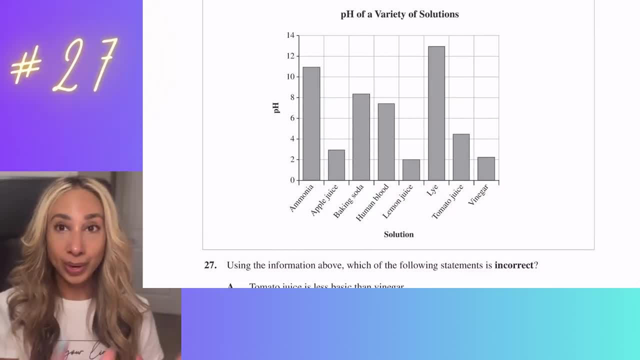 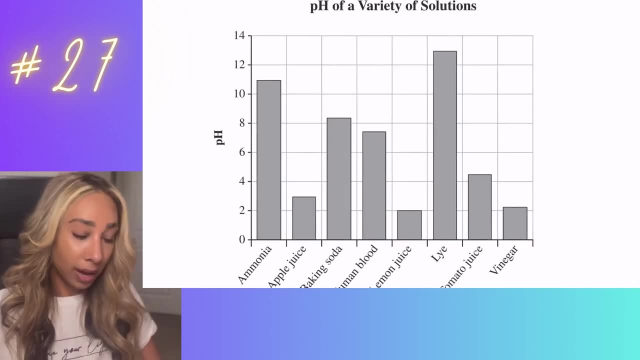 with just the pH, Okay, 27.. Let's look at the graph and then I'll talk about the wording of 27.. So with our graph here we've got the pH, which is 0 to 14.. So that means anything on the higher. 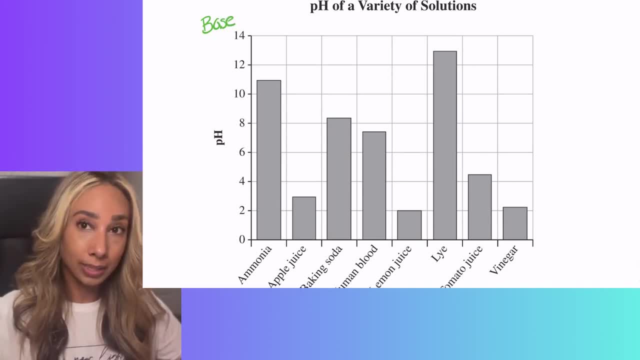 end here is going to be a base and anything on the lower end here is going to be acidic or an acid. So ammonia, very basic. Lime, very basic Acidic components. My most acidic thing is lemon juice. Actually, lemon juice is quite acidic. It's one of the reasons why it's used. 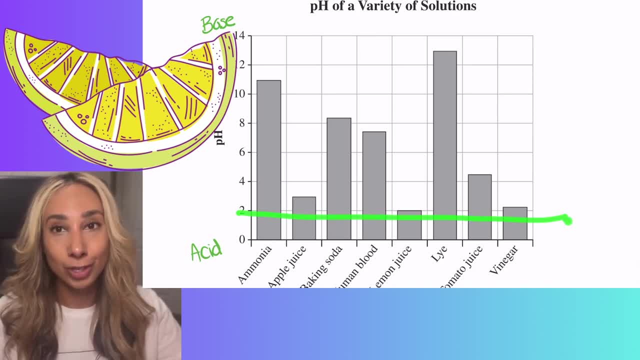 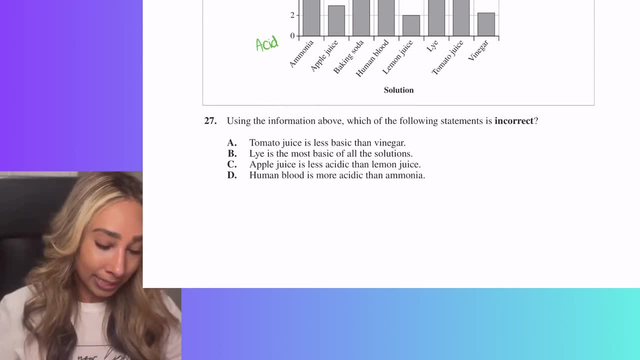 in a lot of cleaning stuff, because acidic bacteria and germs actually can't live in that acidic environment. All right, so that's the graph. Let's look at the questions here. So we need to decide which of the statements is incorrect. So we're looking at the question here: which of the statements 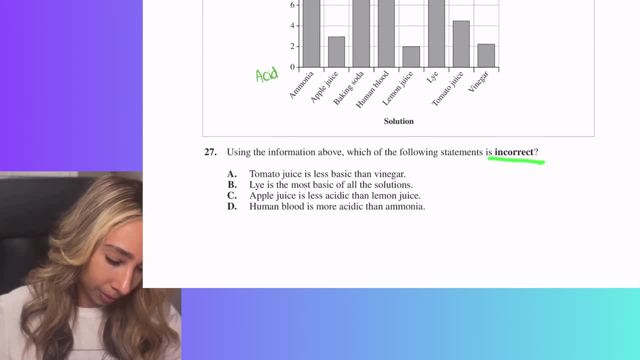 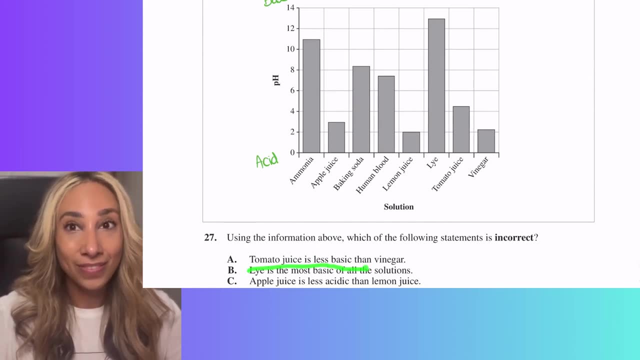 is incorrect. So we're looking at the question here. which of the statements is incorrect? So we're looking for a false statement. let me put it so we can see everything here. okay, tomato juice is less basic than vinegar, so they wrote that in a very interesting way. I'm going to go ahead and change. 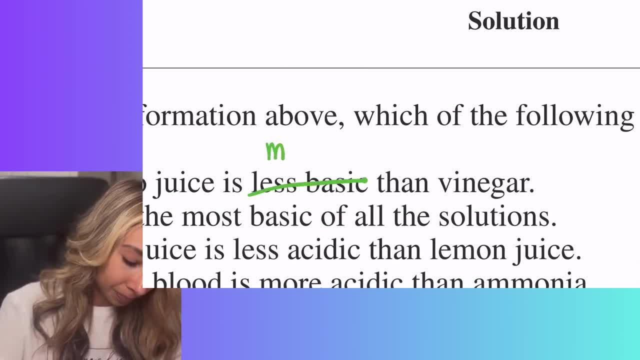 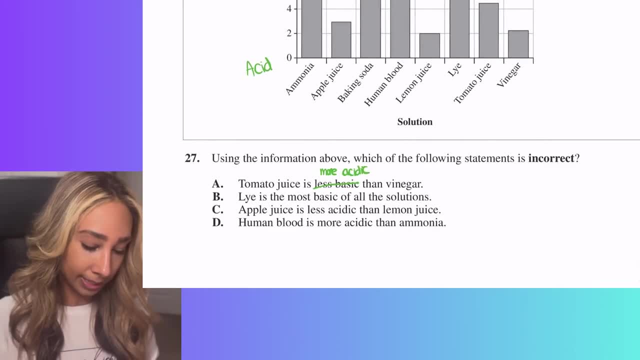 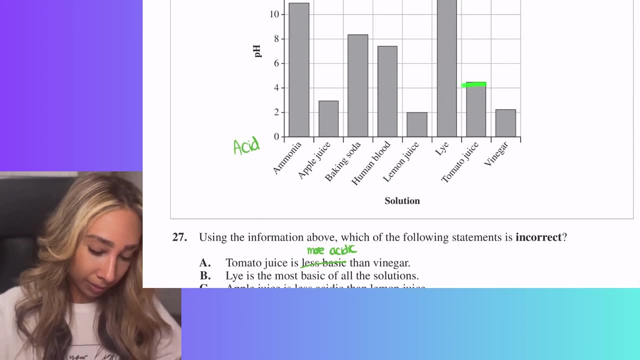 that to say more acidic. that works for my brain. if the less basic works for you, go ahead and keep it that way. so let's see, tomato juice is more acidic than vinegar. okay, here's our tomato juice and here's our vinegar. no, actually, uh, vinegar is more acidic, so this one very well could be. 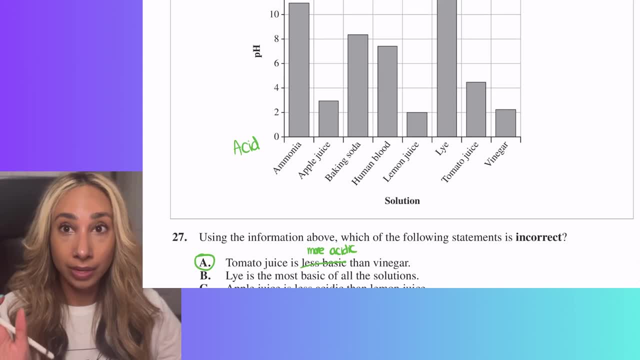 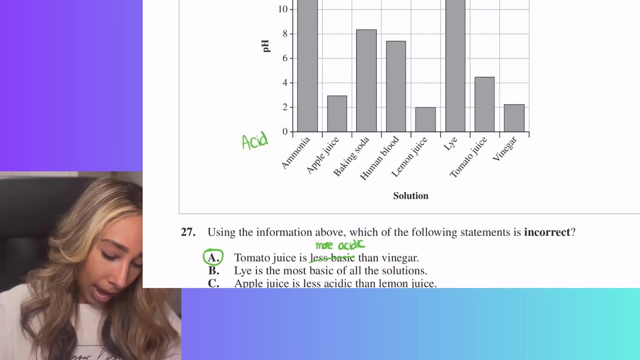 your incorrect response. but again, let's always verify everything, just to be sure. lye is the most basic of the solutions. yep, that checks out. apple juice is less acidic than lemon juice. apple juice is less acidic, so it's less acidic. then that means the lemon juice is more. 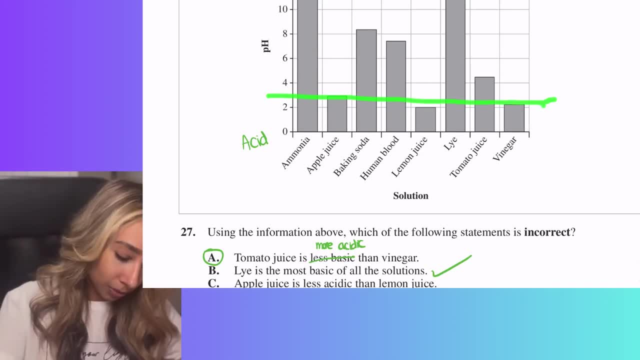 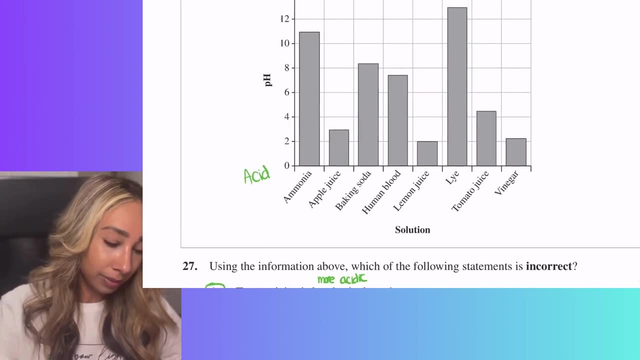 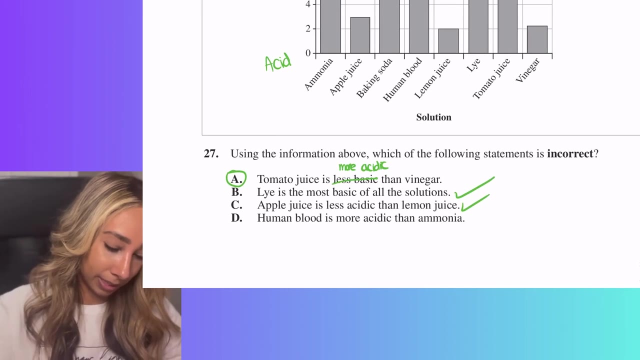 acidic. well, we confirm that. we said our lemon juice was the most acidic. so that one checks out as well: human blood is more acidic than ammonia. well, if I remember correctly, ammonia was our one of our highest ones. there's ammonia and there's our blood, that one works. ammonia is definitely more basic, so in this case, our 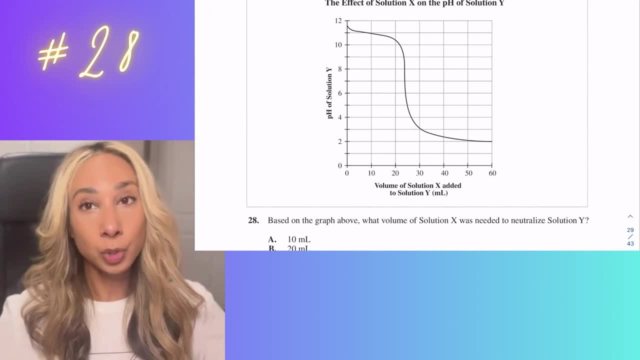 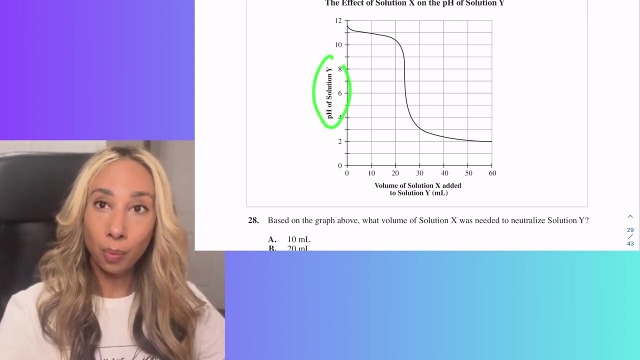 incorrect response is going to be eight. okay, number 28. so this type of graph, um, you may or may not have seen it before. it does kind of start to connect to more grade 10, grade 11, science. but let's see what's happening here. we're looking at um, the ph, again on the y-axis, and we 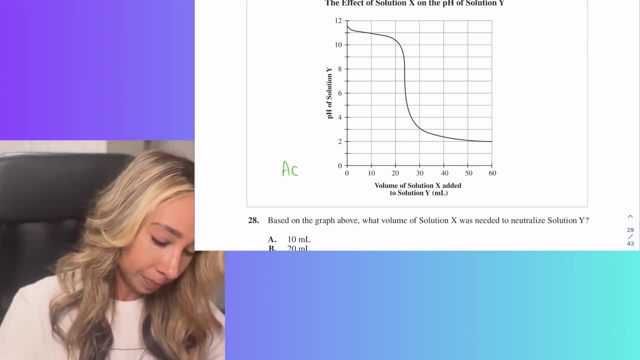 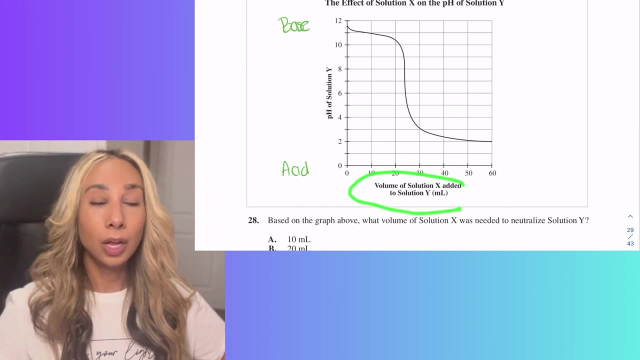 can see, we've got a very low ph. so that's going to be our acid again and this is going to be our base. so what's happening is, over time, we're adding a solution, so we're starting off at a very high ph and we're adding something that at the end we end up in a low ph. so one of the things that can 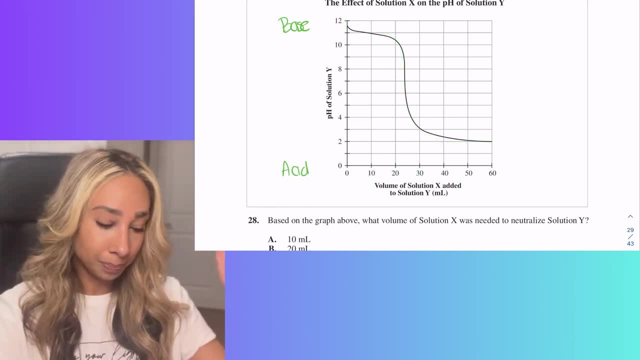 really account for. that is, if we're starting at something basic and we end up with something low. that means we're adding an acid over time. that's how we went from high to low, so that means this portion here. that's probably going to be the part where it was the most. 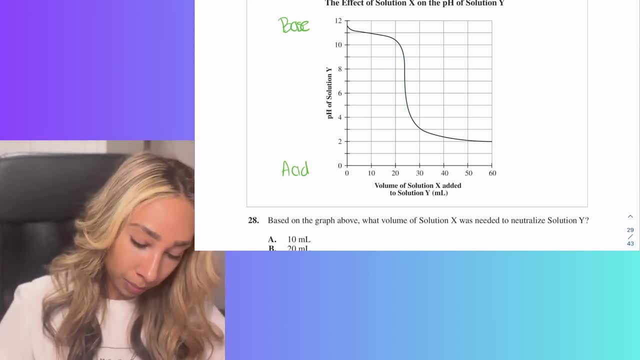 neutral. so what we can do is, in our question we want to know what volume of solution x was needed to neutralize. so now we know for sure it's a neutralization reaction. so the way this is going to work is we're going to find our neutral ph on the y-axis. so the neutral ph is going to be about. 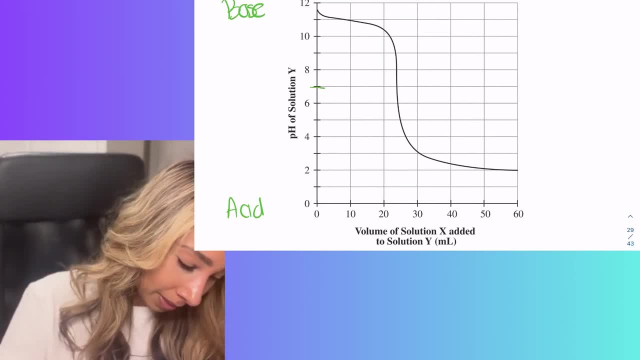 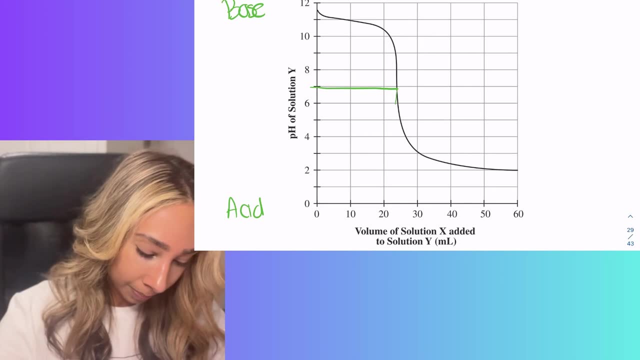 seven. now it's going to be about somewhere, i would say about seven and a half. so we're going to find about there and we're going to hit that graph. then what we're going to do is check the volume that corresponds to that point that i just highlighted. well, that's going to be to me that. 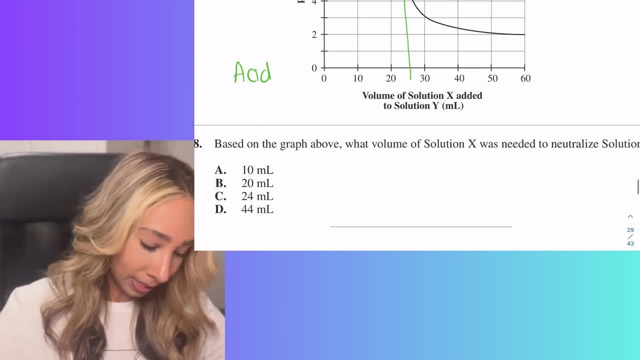 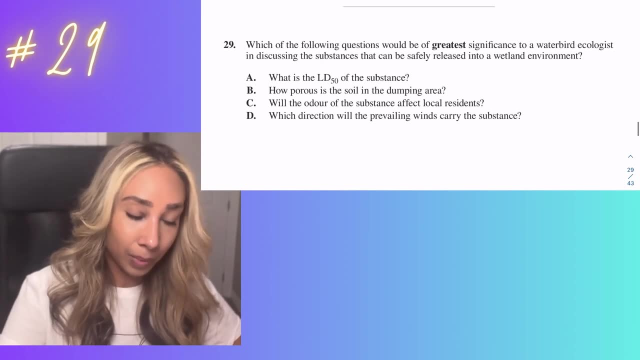 looks like mid-20s, so we're looking for an answer that's going to be in the mid-20s. we've got one, we've got 24, so that's going to work. okay, number 29 for this one. um, i'm going to read it out loud: 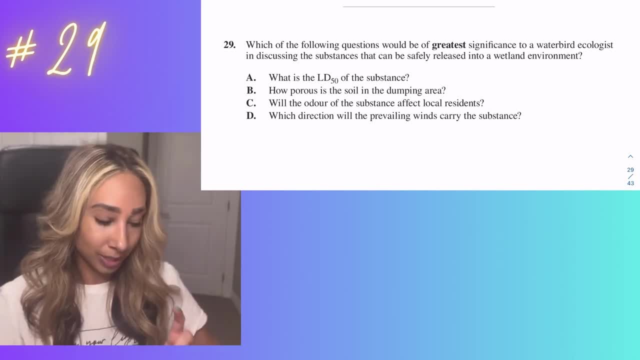 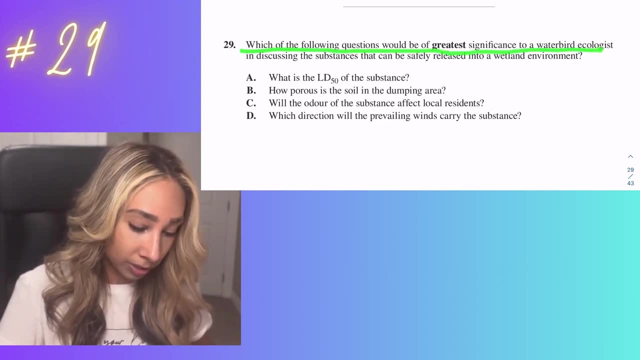 and then it's really only pointing to one kind of concept out of these options that's going to work in my opinion anyway. which of the following questions would be the greatest significance to a logical, ecological ecologist in discussing the substances that can easily be safely released into? 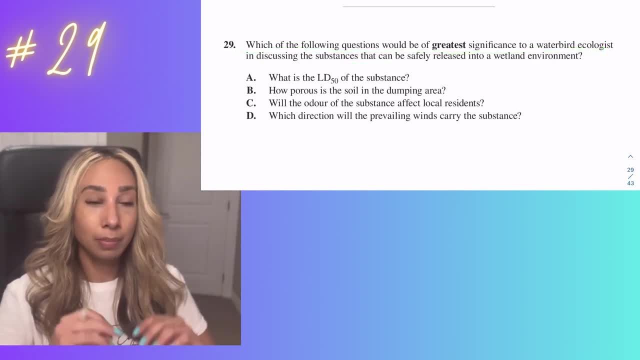 the wetland environment. so if we're thinking of things that can be released into the wetland environment, it needs to be safe, meaning it has to be low quantities of a toxin. but if it's in a wetland environment, that means there's organisms and water that um need to make sure that they. 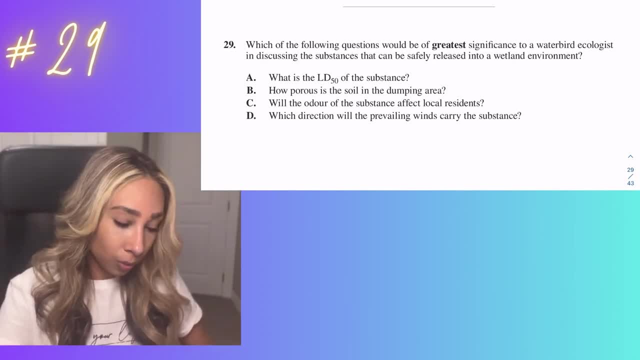 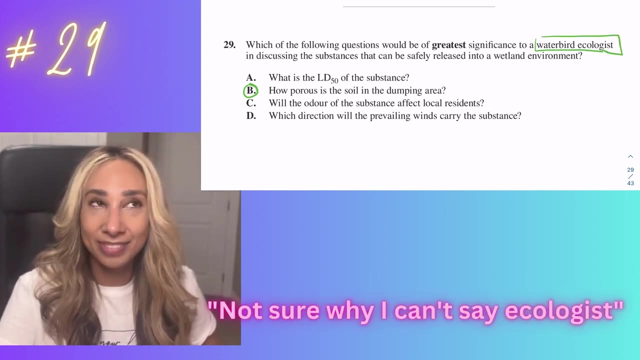 don't react to those unhealthy toxins. so, thinking about the porosity of soil, yes, that is an impact, but it's probably not gonna be of concern to a water bird ecological ecologist. to a water bird ecologist, nope, can't do it to a water bird ecologist. there we go to a. 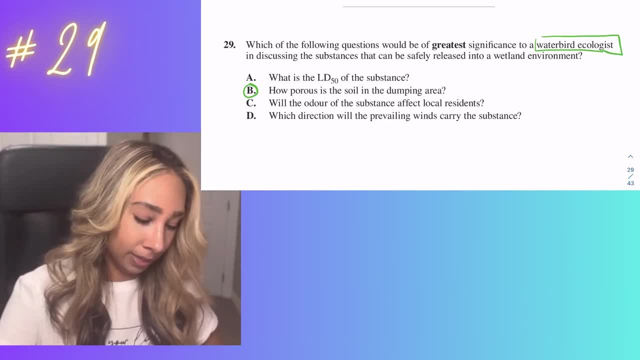 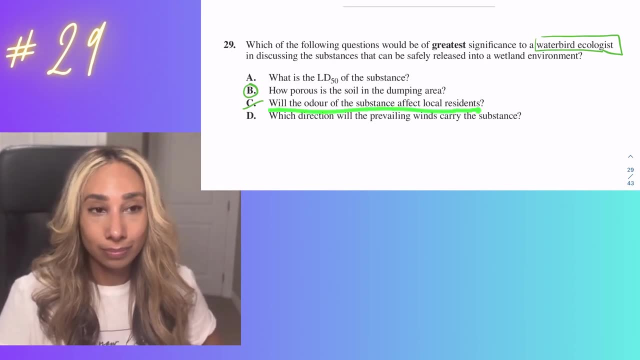 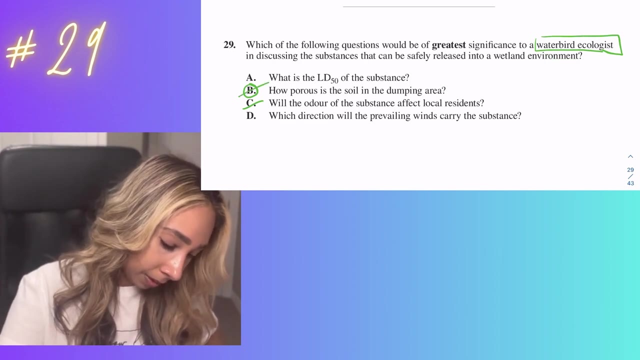 water bird ecologist. um, the odor isn't really gonna the the residents. sorry, let me read the statement again. will the odor of the substance affect the local residents? again, we're talking about a specific system here, so that one's probably not gonna work. um, and the direction? 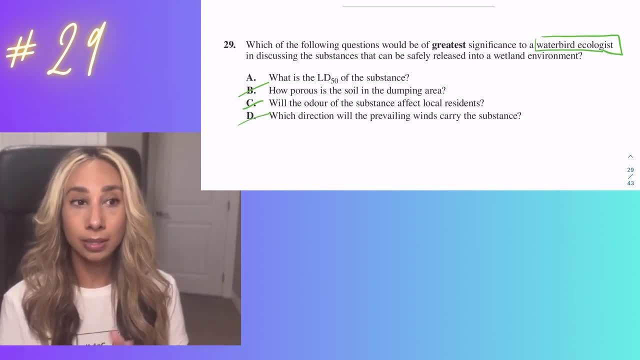 of the winds again, that's not gonna work. what's really gonna be of importance is that toxicity with the ld50. so the ld50 is like. i'm gonna put the definition up there. it's the lethal dose that um can harm an organism and normally we want half of that if we are going to expose an organism to. 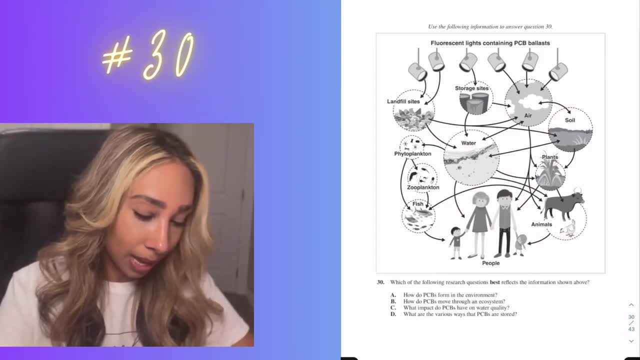 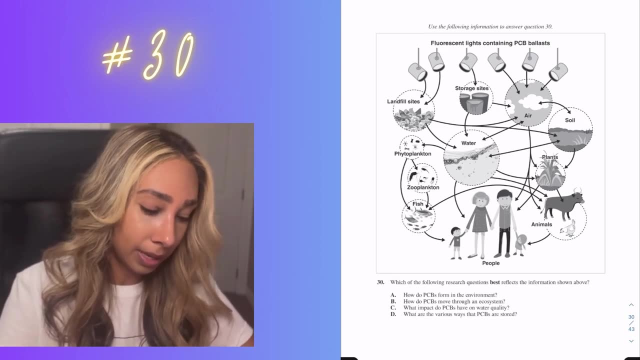 that, okay, number 30.. so what's happening with number 30 is we have fluorescent lights and they contain bcp. so let's see what's happening. some of these end up in landfill sites. they end up in the water. so in the storage sites they're going to end up in water, which affect 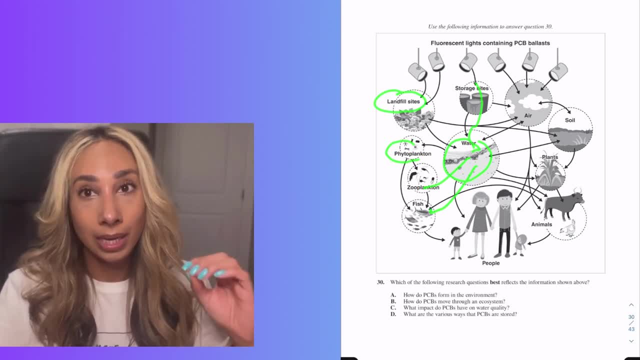 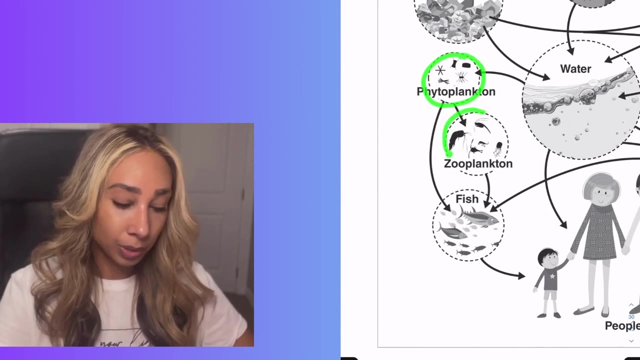 the plants, or excuse me, which affect the aquatic environment, keeping in mind that anything that affects the water is going to affect us. so remember, there's that um concept of biomagnification, right? so in this example, here, the phytoplankton gets exposed to the toxin, but the zooplankton have to eat more phytoplankton to survive, meaning the zooplankton get exposed to more toxins and then the fish eat lots of zooplankton that are eat phytoplankton that are also um exposed to those toxins. and then the human- probably the whole family, not just the kid, um also. 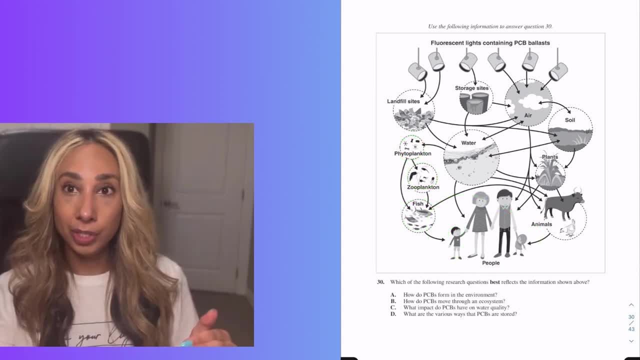 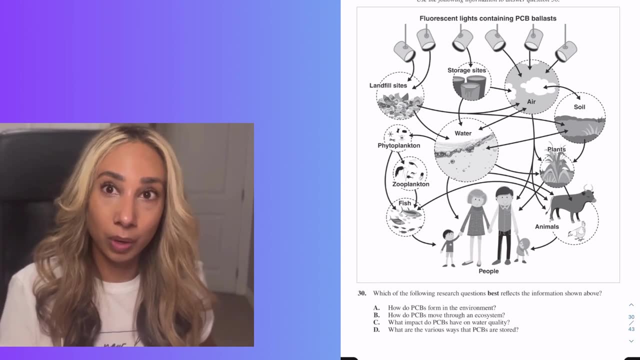 get exposed to the toxin, right? so as it goes through a food chain, the level of toxicity accumulates, right? um, it's one of the things that, um, you might want to think about, kind of what, where your food's coming from anyway. so we've got landfill sites, toxins- we know things end up. 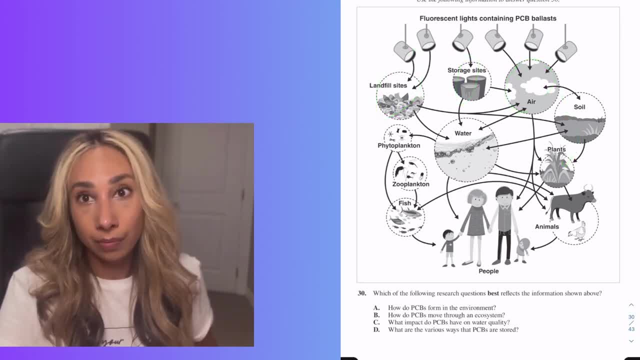 in the air and all these toxins are going to end up in parts of our ecosystem. so the question's asking what would be the best research question that that would um illustrate the information about. so they're asking: how would you assess this as a research question? so